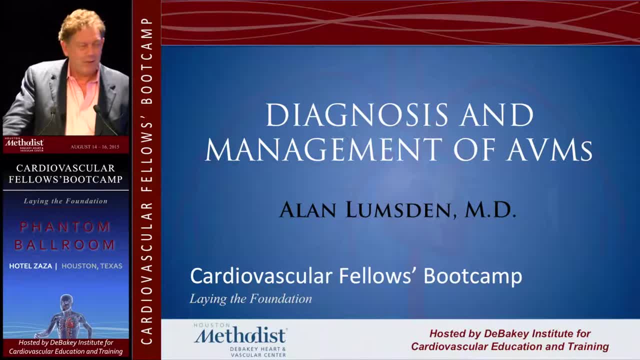 them out, got the phones in the ears and played some music and said: randomize my legs. So I had no idea what was done until I took the bandages off the following day. One side looked normal. The other side is black and blue, literally from ass to ankle. at that particular 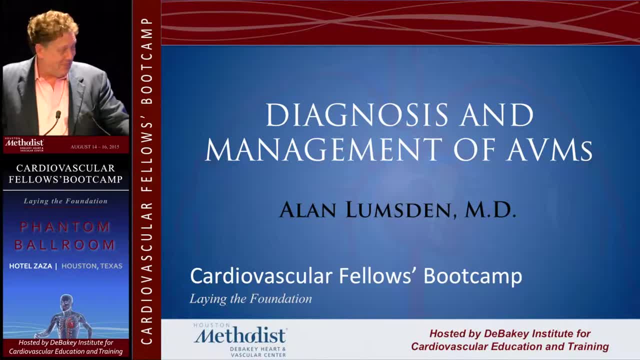 point in time, And that was the end of venous laser. So I had the opportunity of hearing a debate at VIVA one year between one guy who was an advocate for venous disease and Manny Mehta was the advocate for RF ablation, and they had no idea what they were talking about. So I got. 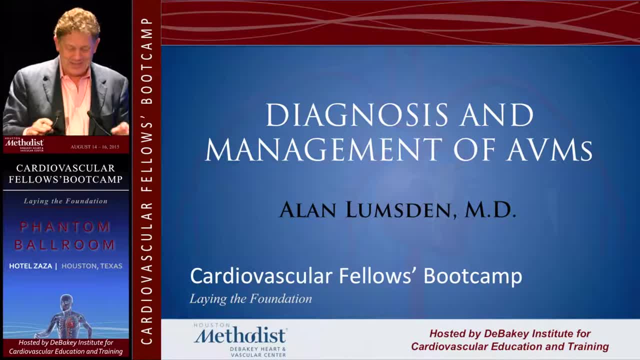 up at the podium, followed them and said: let me tell you what the real answer is in this situation. So that's the answer: Don't get the laser. The reason they use the laser is because it's cheaper for the guys to buy it in the office. So see that $7,000? They're. trying to take all of that home, based about a $3,000. So that's the end of the laser. So I had the opportunity of hearing a debate at VIVA one year between one guy who was an advocate for sonocächlich. They're trying to take all of that home, So they. 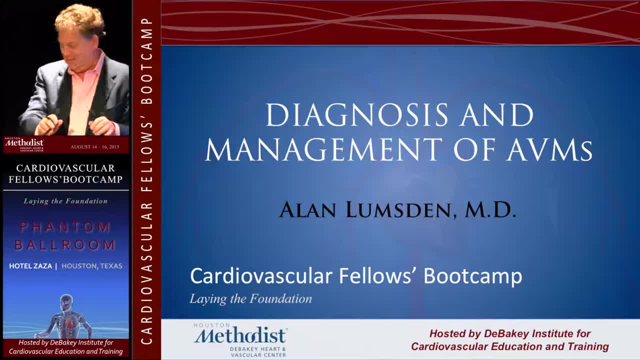 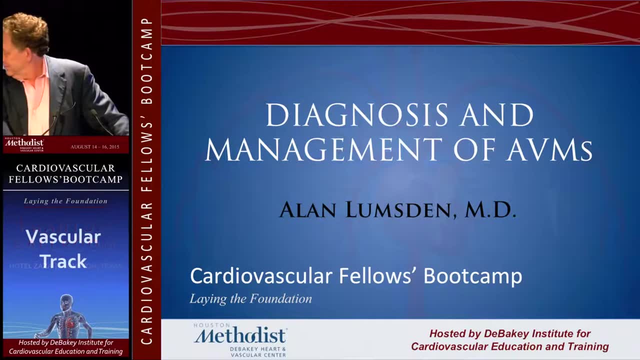 get all of that home, based about a $300 laser versus a $1,000 catheter. Isn't that the truth? That was a different wavelength. Oh yeah, They changed the wavelength all the time. All right, The fourth to시고. 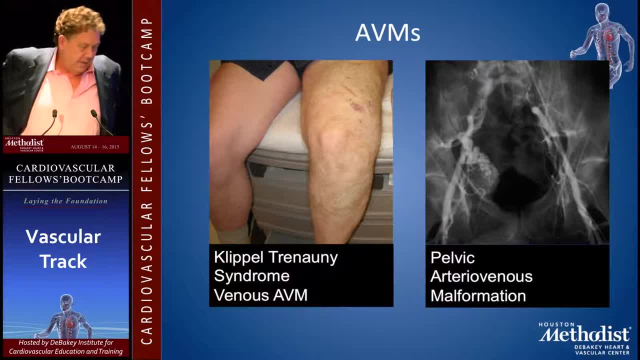 All right, So I'm going to talk about AVMs. AVMs is actually something we are very interested in. We run an AVM clinic And these people need a home, because this is kind of like MEN-1 syndrome for vascular surgery: You're never going to cure it and they're always coming. 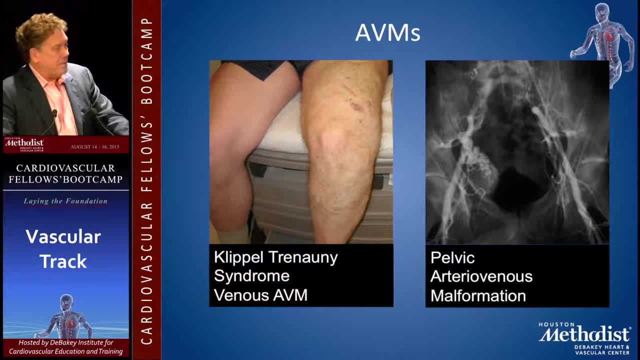 back, and so it can manifest in a variety of different ways. So this patient on the left is a patient- still a patient- of mine: big swollen leg, he's got clipper-Trenony syndrome, he's got absent deep venous system and he's got venous. 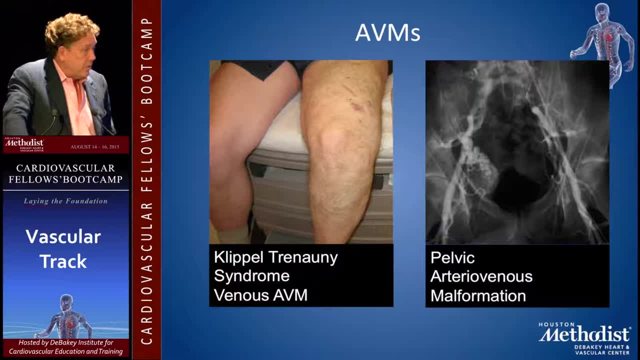 malformations and he has a sciatic vein. aneurysm, which sits on top of the sciatic nerve, causes him a lot of trouble, but so far we've stayed away from that. The patient on the right, as you look at it, has an arteriovenous malformation. 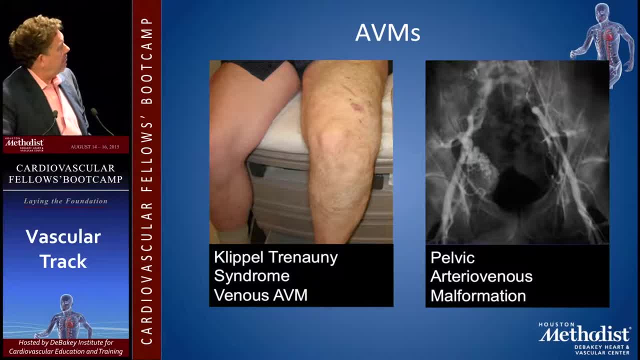 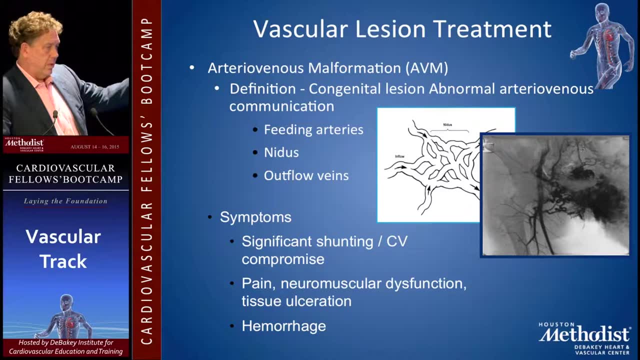 and so it starts off with all of these different classifications which you're gonna come across. but let me try and simplify all the stuff for you. There are arterial and venous malformations, which is truly mixed arterial and venous flow, and there are venous malformations, and there's all. 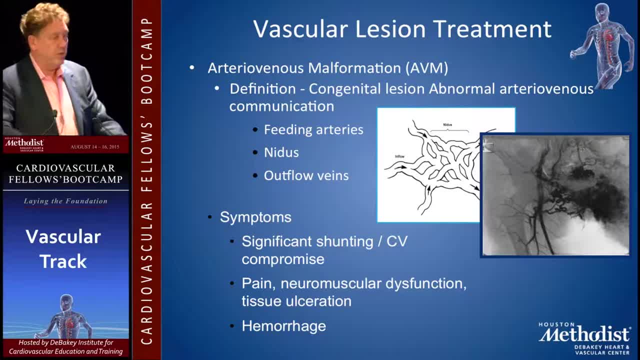 kind of gradations, basically between the two. The approach to true venous malformations is very different from an arteriovenous malformation. Venous malformations you're gonna treat with sclerotherapy, foam sclerotherapy. 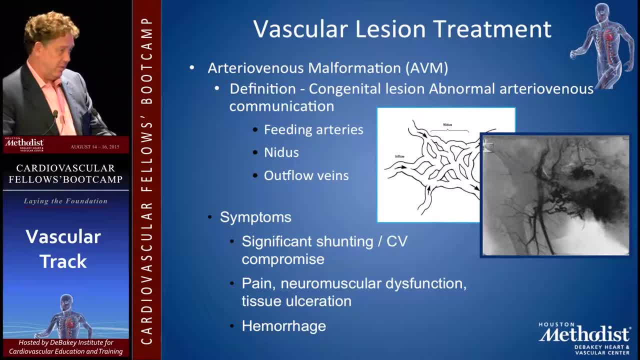 and you're go to use image guidance to actually get access to those arteriovenous malformations you're usually going to treat from the arterial side at least first and you're going to try to get as far into it. Everybody talks about the nidus. Everybody talks about it. I have 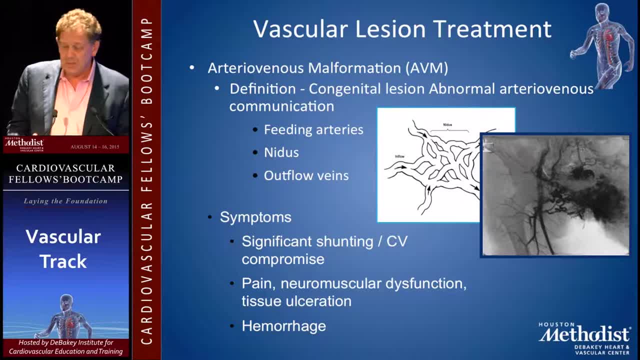 no idea what a nidus actually is. It seems to me that a nidus is get the catheter as far out in the middle of that thing as you could possibly get, but I've never seen a little symbol which says nidus yet, because there may be multiple niduses or nidi Do. 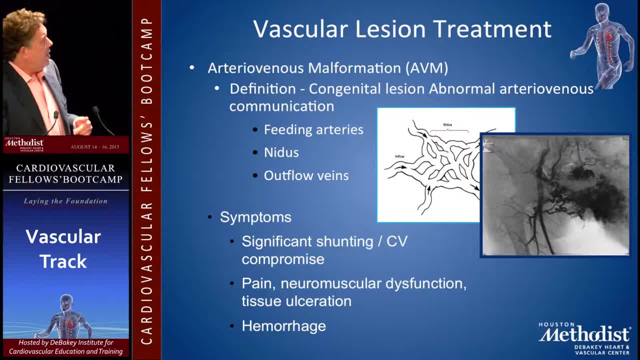 you think nidi is the appropriate way of saying this. So it's impossible to say how these things present, because it really depends upon where they are. They may be in the extremities, They may be in the face, They may basically be deep inside the trunk, and so the manifestations. 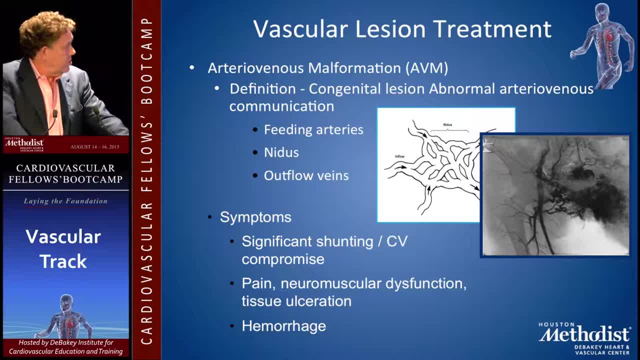 are really based upon where they are localized to. Sometimes there is disfiguration, There's a swelling, Sometimes there's pain because it's compressed in the nerve, Sometimes there's bleeding and it erodes out through the skin, and sometimes there's shunting Everybody. 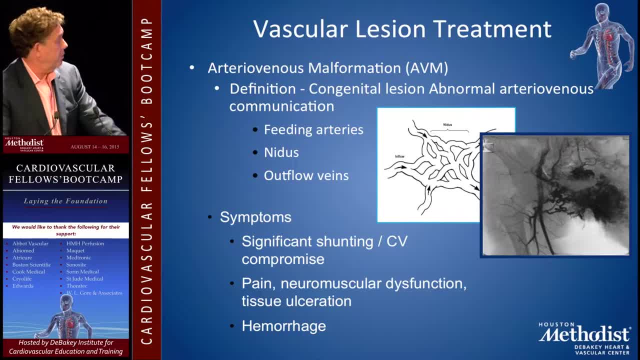 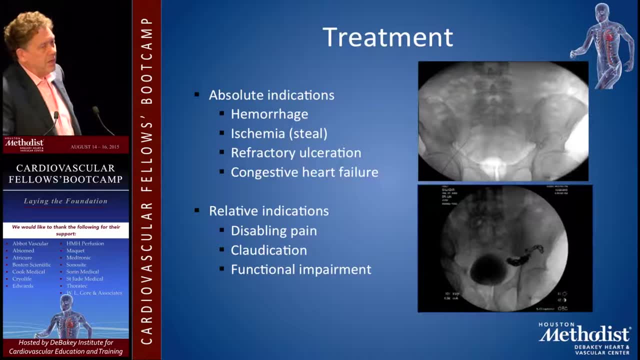 talks about this. This is pretty uncommon to see heart failure result with shunt, but it does actually occur. So very heterogeneous in terms, basically, of how they present. So when you find them it doesn't mean to say you've got to fix them. Some of these patients live with them for 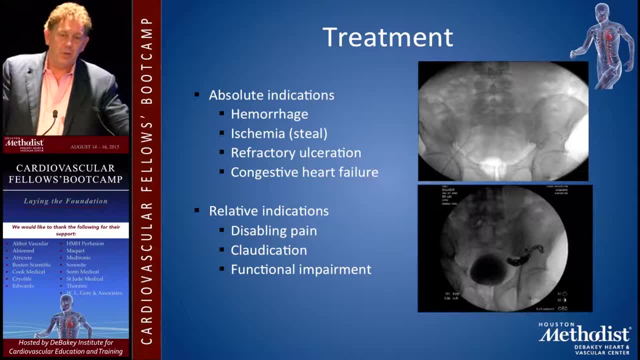 a long period of time. Certain things tend to accelerate their growth. Pregnancy, puberty, trauma are the sort of things that seem to be associated with acceleration of the progression of arteriovenous malformations, And so there are absolute indications for intervening on 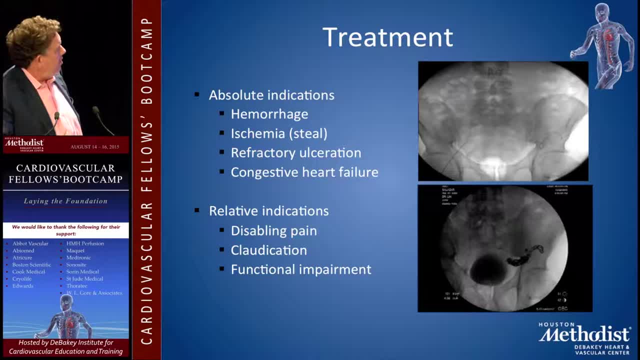 them and a few relative indications: Hemorrhage, ischemia from Steele syndrome, refractory ulceration. Sometimes they're associated with Steele to the point they can get claudication. That's pretty uncommon. It's usually functional impairment from local compression. that's going to take. 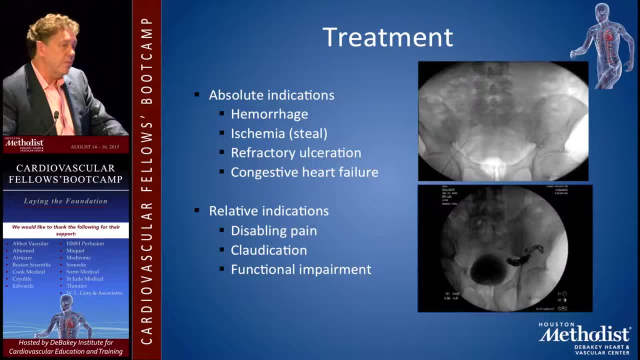 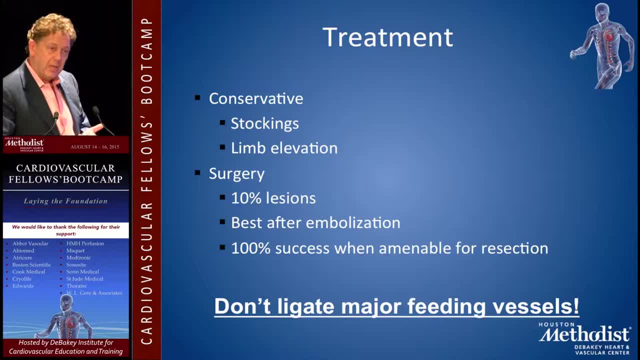 localize it in terms of what structures it abuts up against. And again, the things that make these non-resectable is usually because they're in and around nerves, But sometimes they're localized, and these are the few that you can actually cure by taking them out. 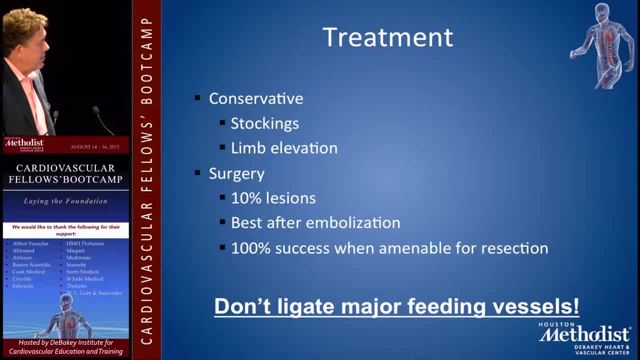 And occasionally, if they're big, you want to pre-embolize them before you actually take them out. So it's probably the only time that you're going to actually be able to take them out. But don't ligate major feeding vessels. For example, we saw a patient who came in 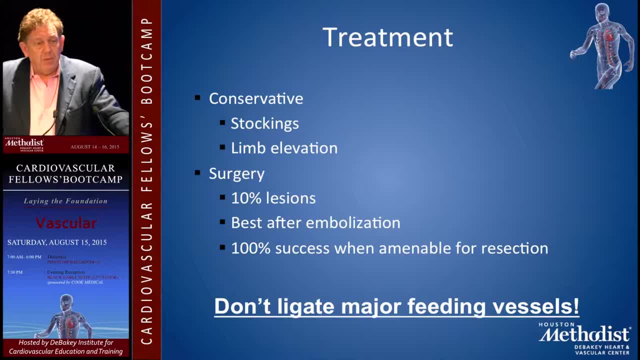 with vaginal bleeding because she had a pelvic or tibia small formation And what had been done was a surgeon had explored her and ligated the internal iliac artery. Fortunately, we weren't even very good at that, because we actually managed to get back in through that. 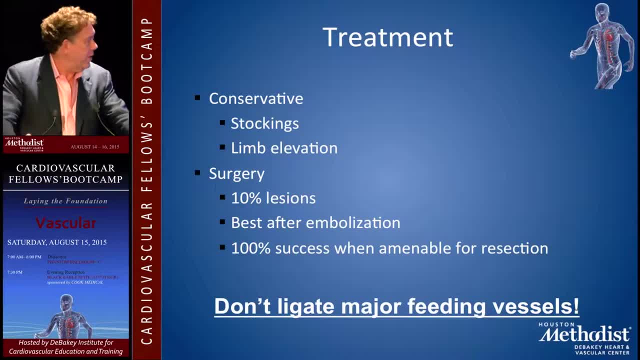 ligation angioplasty, open it so we could get access down into the pelvis. So it's surprising how many times you see blood vessels that surgeons have ligated but they haven't actually managed to occlude them. I actually saw. I believe I saw that from one of your partners. 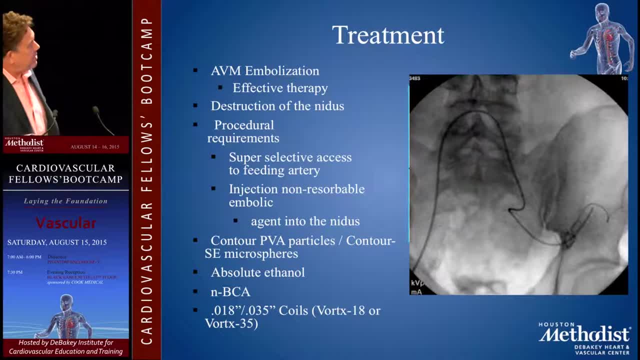 many years ago, Mike, Many, many years ago, Anyway. so what's the mainstay of therapy Let's talk about- No longer with us. Yeah, I know that The mainstay of therapy for tibia venous malformation is super selective catheterization, And so. 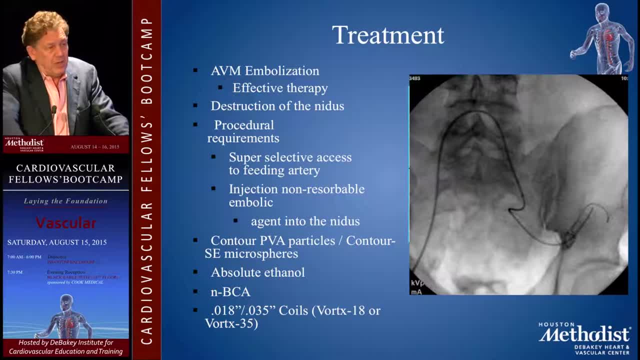 if you're looking for a technical challenge, this is kind of one of them. It starts off by doing angiography, which looks at the feeding vessels. You need to know which vessels are coming into it And you need to know when you block off, let's say segment A, you're. 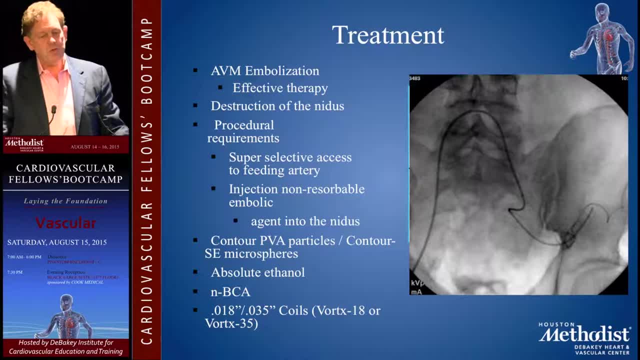 getting blood flow changes and you may get outflow through segment B. So you're always trying to evaluate: if I start putting stuff inside this AVM, where can it end up. And often as you start blocking off the AVM, so the way the blood flows through the AVM changes. 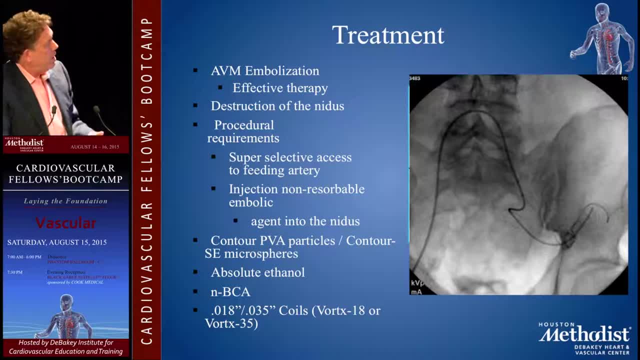 So you're continuously looking to see how it's changing, because non-target organ embolization is one of the complications really for what you're trying to avoid. So the principles are: map out the blood supply, Use it from the arterial side, Understand what the collateral. 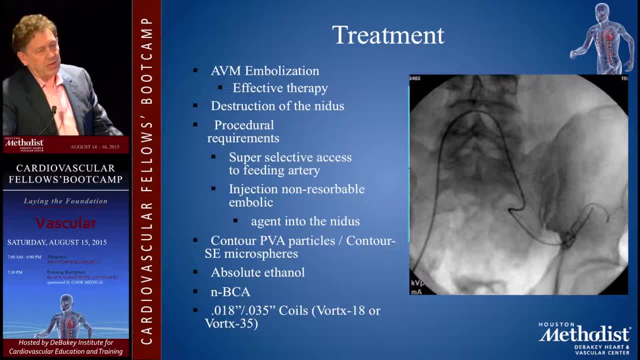 pathways actually are, And then basically to get super selective catheterization. So this is where you're going to need to know about sheaths to give you stability, Five French catheters really to get you out into the smaller blood vessels, And then micro. 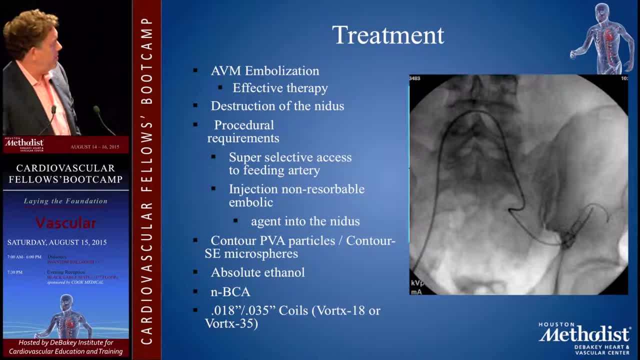 catheters that are going to go through the five French catheter to get you way out into the middle of these things, And so typically what you again, it's not usually caused. The whole concept now has moved towards flow-directed embolization And there's really only two. 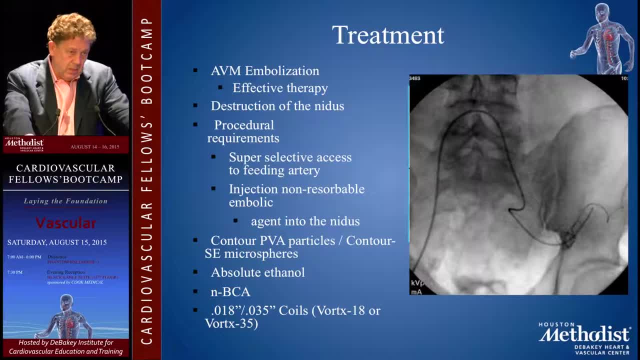 things that are out there which you're going to use for that, And that is onyx, which is largely supplanted all the other things. So onyx and glue. Glue is something that is not for the faint of heart, because you can glue these catheters in And so you've got. 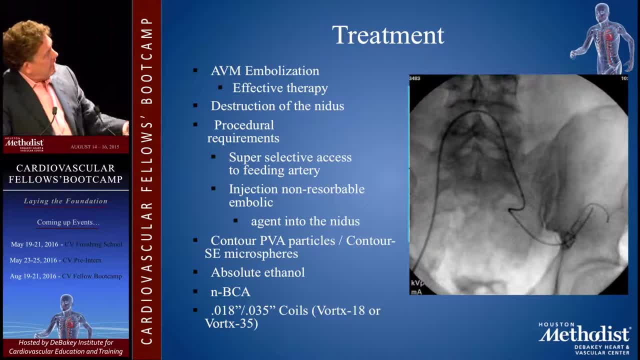 to understand the speed at which blood is flowing through this. The advantage is that glue gets fairly far into the AVM, but that means it can also come out the other side of the AVM. So most people have now gone to use onyx, which is more like lava. It hardens. 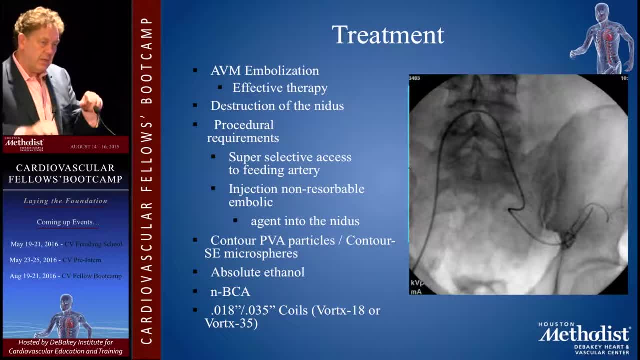 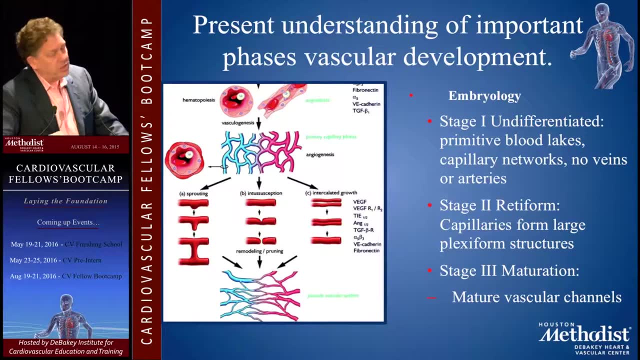 slowly, And as you push on the back end of the onyx it pushes the onyx further out into the arteriovenous malformation, So it will get you much further into the AVM, Thank you. Then you can actually do otherwise. So again, there are all these different. 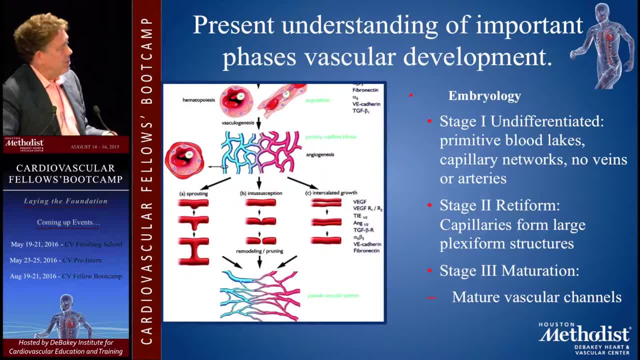 classifications based on embryology. They are irrelevant to treating these patients. It really comes down to where is the AVM? Is it arterial? Is it venous? If it's purely venous, you're not going to do any of the stuff I've just told you. You're going to. 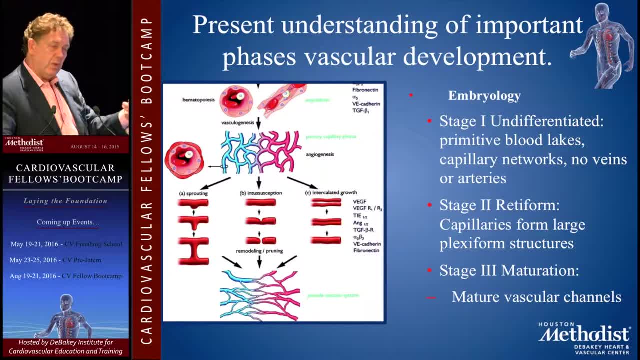 treat it more like big varicose veins, But big varicose veins. you can't put enough tetradecyl sulfate on, So you foam it up. You mix the tetradecyl with air, So it foams it up And 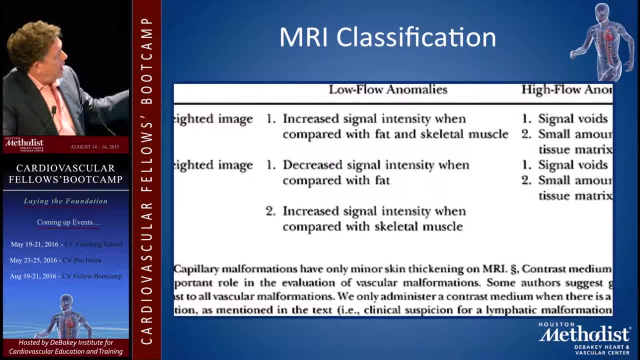 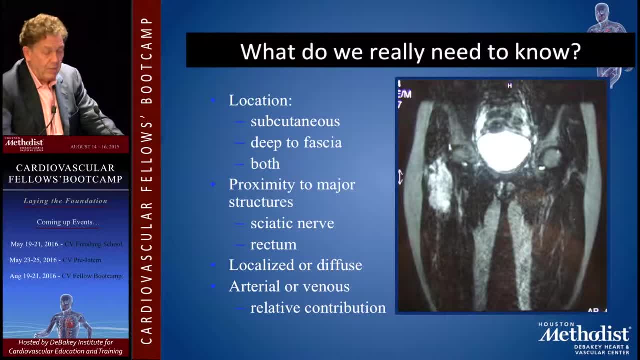 it's those bubbles that will actually fill the arteriovenous malformation with the onyx. So this is a very important situation when you're embolizing it. Again, talking about MR is what we kind of use to characterize these things. This is an example of an MR. 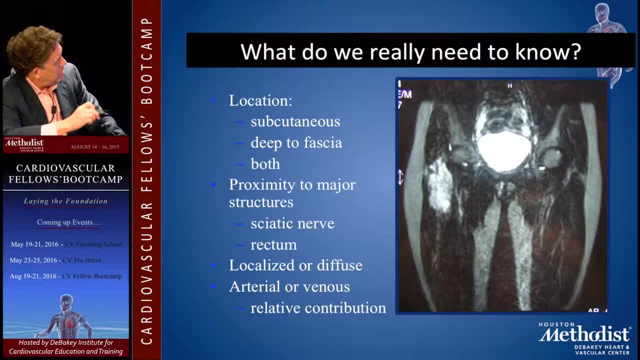 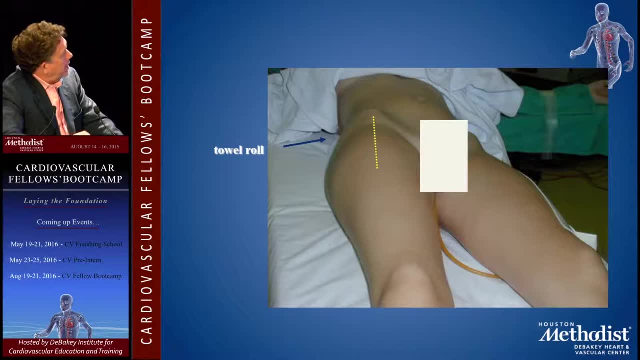 where you have this big signal void in the patient's AVM. Now, this was remote from her femoral nerve And this was a situation where we opted to go ahead and actually operate on her. So this is a young girl She just presented with pain, slight swelling in that. 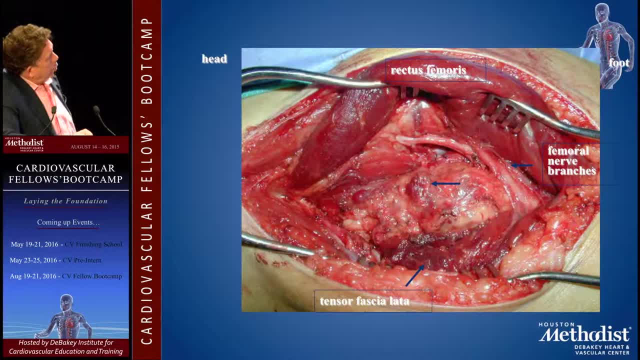 area And that was the MR that you actually saw, And so what we're exploring basically, the rectus femoris has been taken medially. This is the big AVM that you've got in this big cavity. You're separating all the branches. 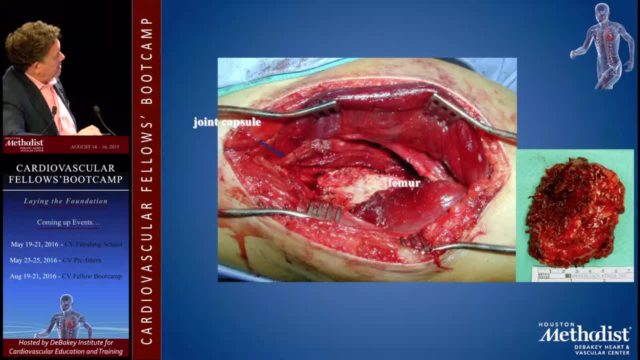 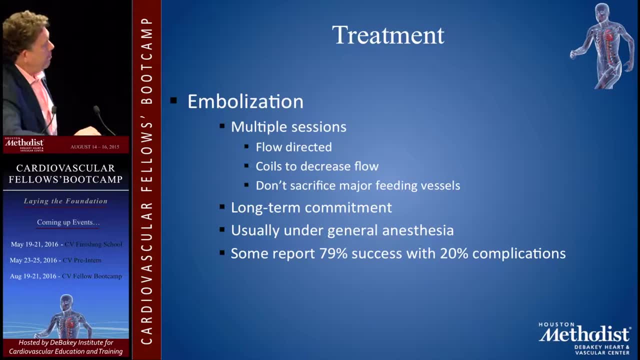 of the femoral nerve off it And we actually managed to completely excise that. It leaves a bit of a hole which we drained, which she subsequently healed up very nicely And she was pain-free. But that's the minority. Most of them are going to be treated with embolization. 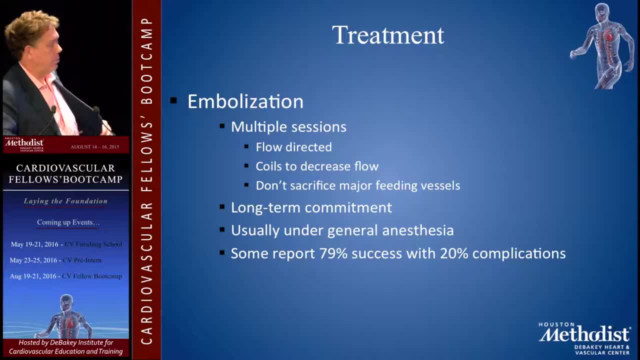 Not one episode of embolization, multiple episodes of embolization. How could you have embolized that? Could you have embolized it? Yeah, that would be pretty hard to embolize. I'm not sure you could, Although I tell you. 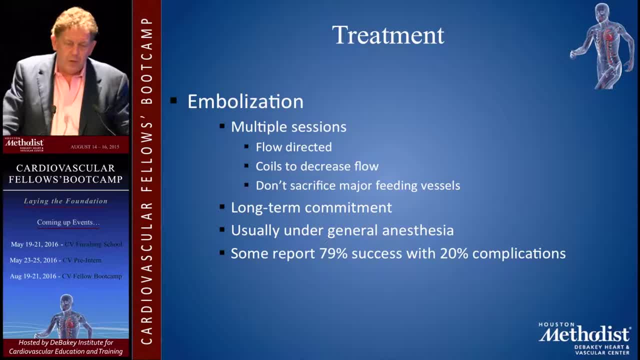 what one of the things. We have worked a lot with our interventional neuroradiologists And I would really advocate that, because they have techniques that we have learned from, For example, direct percutaneous embolization of these things, And we learned this from how I had a patient with a giant. 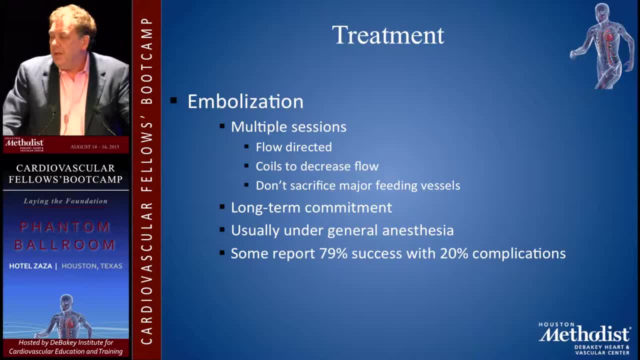 carotid body tumor, which is kind of like an AVM actually, And we were going to embolize this transarterial And as you did all the different injections, you could see that flow was coming out the opposite side and going into the vertebral artery And it really felt. 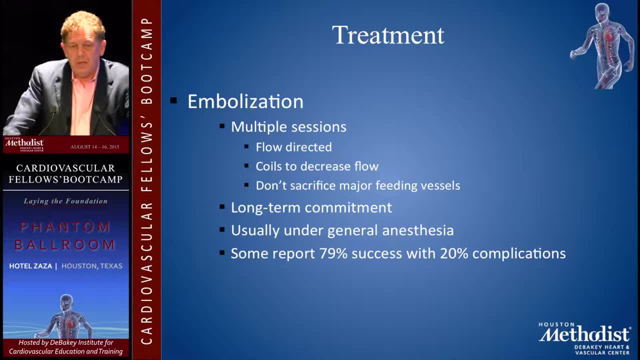 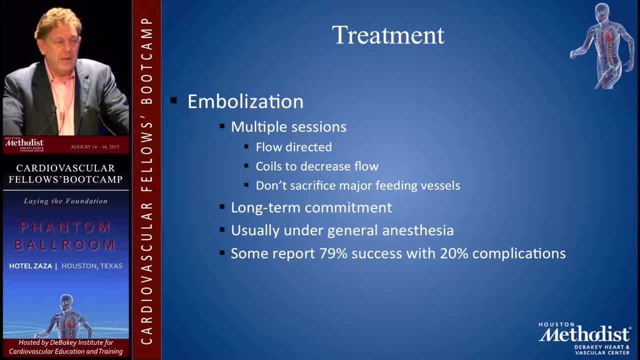 just stick needles in it. We were always taught this is the most vascular lesion known to man And actually we punctured this probably 30 times percutaneously. Every time we did this you got blood return And you were inside the tumor And it looked like an AVM And we embolized it percutaneously. 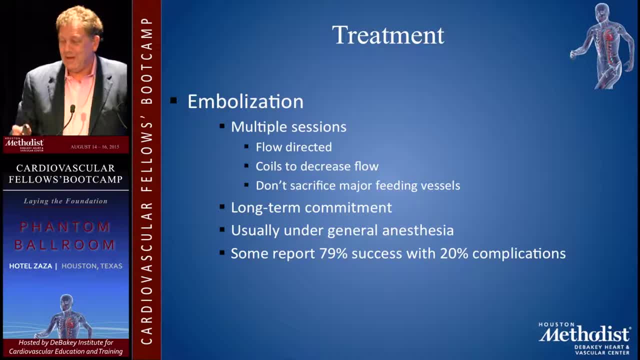 It's the best video And I can't even get it accepted at the Society of Vascular Surgery because they think it's heresy. But there's actually a lot published about that. Now we've actually gone to treating some of the AVMs like that percutaneously. You can actually 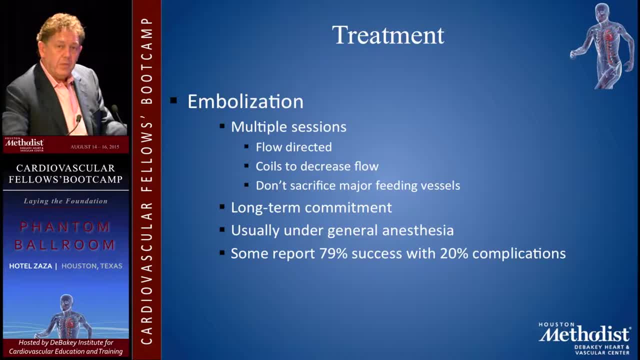 can stick them directly. You pacify them basically by doing the arteriogram. You see it, you map it and then you go ahead and stick it directly and you fill these veins. It's actually a very effective. Do you fill them with alcohol or onyx? Not alcohol, no, with onyx. Alcohol hurts like. 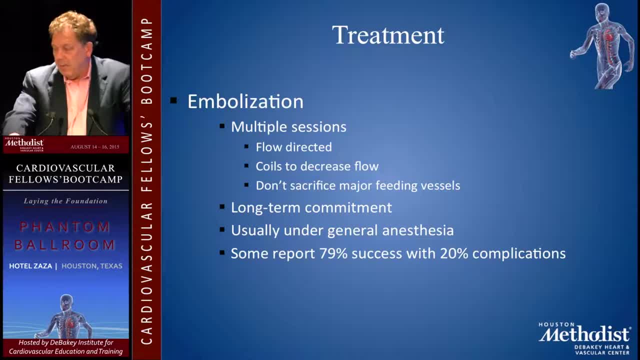 the devil, I'm afraid of alcohol. Alcohol is one of those things that's very effective, you know, at occluding big veins, sometimes more than effective. And so there are those who are devotees. a guy called Wayne Yates, who does a lot of this up in Denver, actually is a devotee. 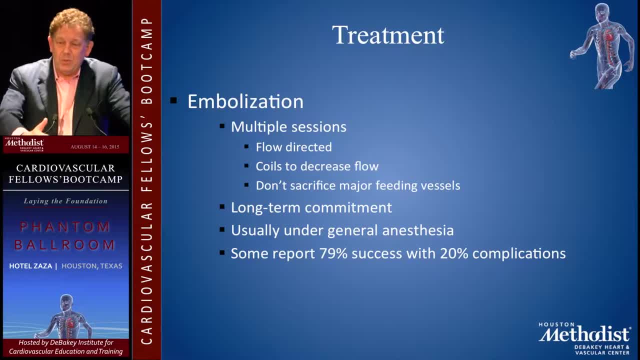 of alcohol, We tend to stay. I would rather do this five times than do it once and have a major complication from it, And so you usually see patients. good things happen slowly when you're doing this. bad things happen really rapidly, So I'd much rather repeat it and minimize the 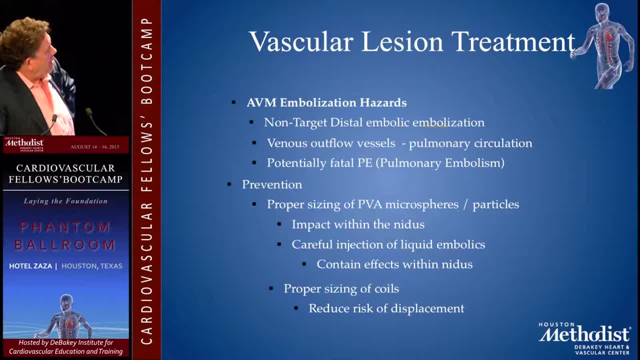 complications. I think we've kind of already really talked about this Again. the hazards are that you block an artery, you keep injecting and the stuff comes backwards into the axial circulation and ends up sweeping down the leg. So you've got to know when to stop. You can get Stuff goes. 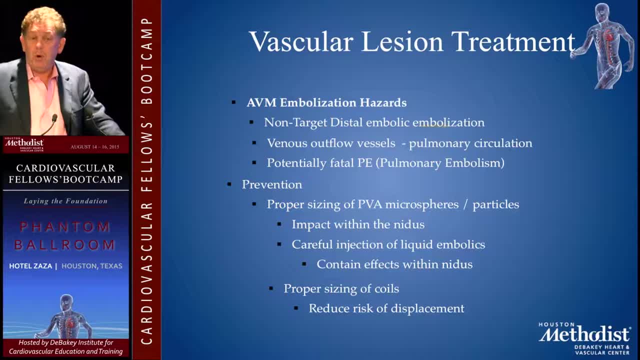 through the circulation comes out the other side, And so you've got things like pulmonary or terevenous malformations. One of the concerns is that you embolize through the AVM and out into the systemic circulation. So stroke is one of the. 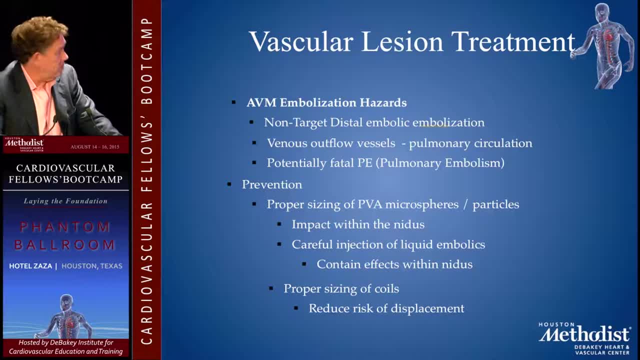 complications that you can actually get from this, And so one of the things we've often done is with Zolt Garami, who does TCD. if there's any question about this, we'll do TCD monitoring. We'll see if. 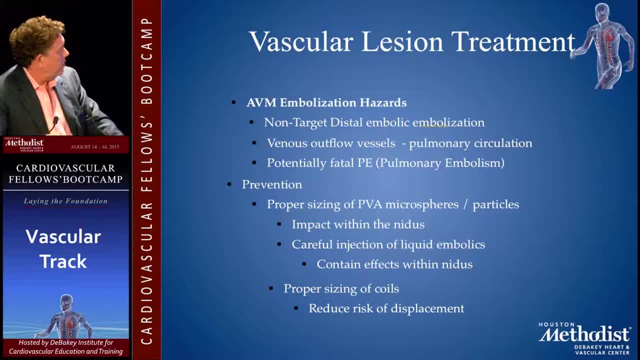 there's any evidence that hits are actually occurring up in the head while we're doing this, we'll stop Things like PVA, microspheres and gel foam- really it's just kind of used to characterize. So if you're going to preoperatively embolize a renal tumor, for example, that's all. 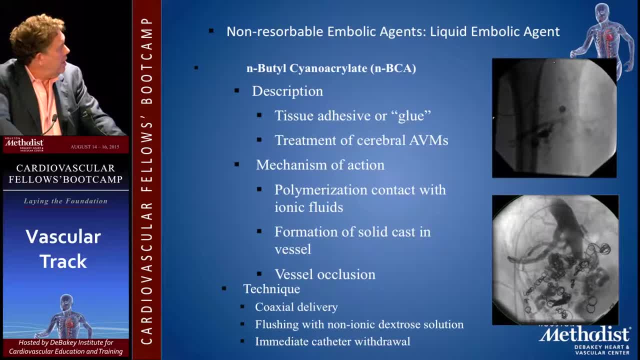 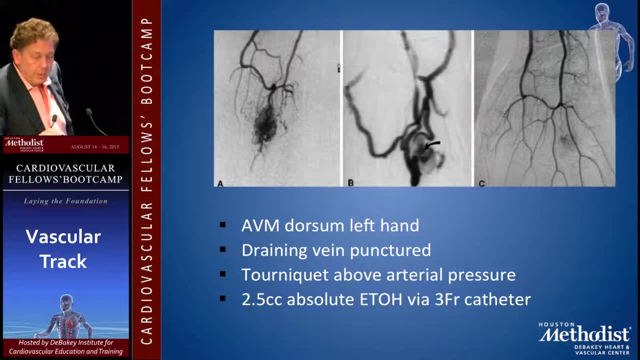 that you need, But for true terevenous malformations it's more in onyx, And this is kind of Well. we'll walk you through this case down at the bottom. This is an example where you essentially unloaded- Let me go back one, Almost unloaded- everything in this patient. This was a patient. 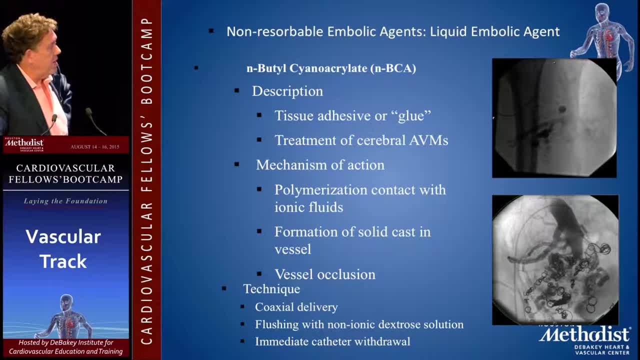 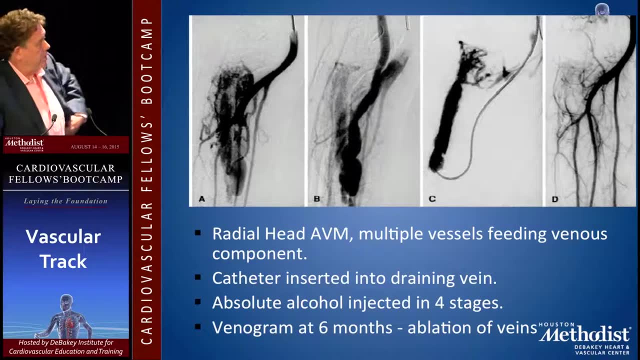 actually who bottom right picture? who was referred from Greece and did have true high flow heart failure from a massive pelvic AVM, And so we used onyx, we used coils. One of the concerns in this patient was there was such high flow through it that the internal 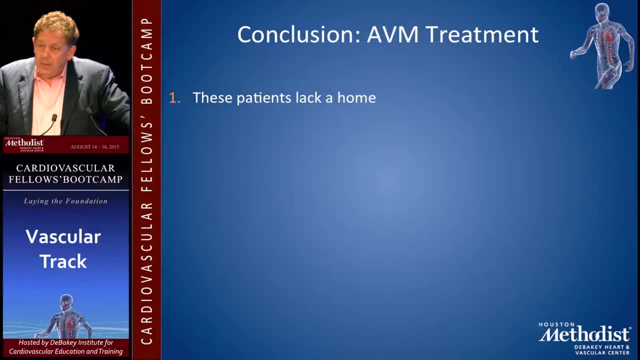 iliac vein was about six to eight centimeters and the right common iliac vein was about the same size. So we were very concerned that shutting down the flow through this would result in a huge DVT. That really doesn't happen. It's more conceptual than it is reality.